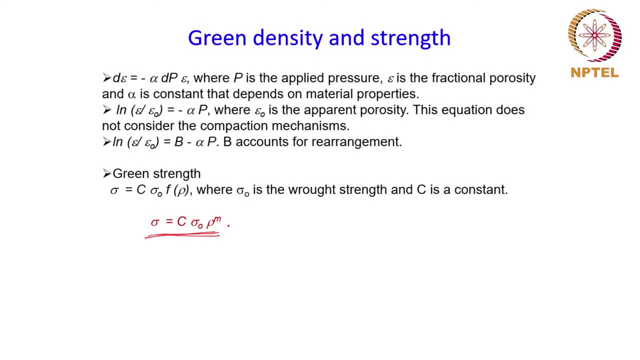 influence on the green strength and the surface conditions also will have a bearing, because this interlocking that happens between the particles will depend on the surface condition. A clean powder surface is always good for interlocking to happen through a cold welding kind of mechanism, and therefore a clean powder will give rise to a higher green strength. 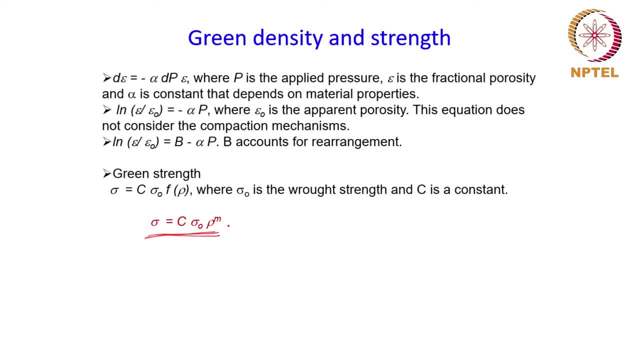 And for the same reasons, when lubricants are added to the powder, it might decrease the green strength because, since there is a presence of a lubricant film on the powder, particles interlocking will be adversely affected and, as a result of that, this particle bonding, which 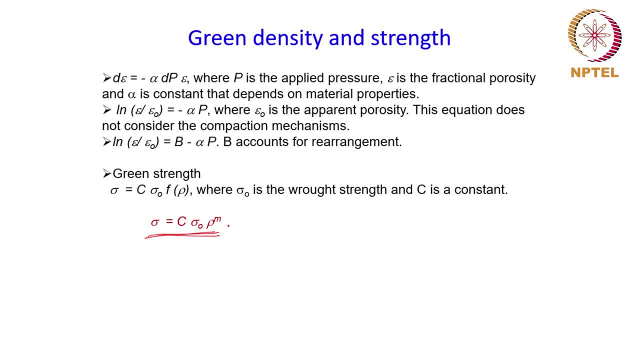 happens by mechanical interlocking, will suffer and as a result of that, the green strength will decrease when the lubricant is present. Now if you want to correlate the green strength with the compaction pressure, then you have to go back to the equation which: 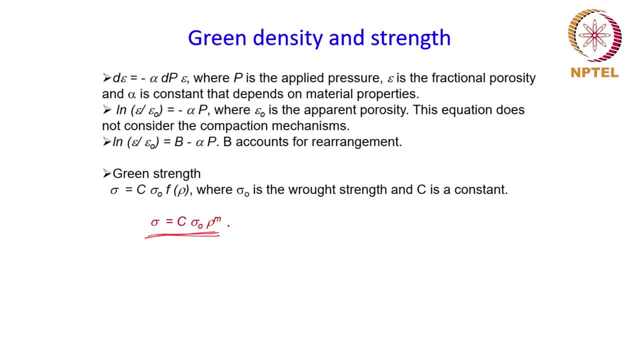 relates the fractional porosity to the compaction pressure. So, if you remember, this is the equation, This we have already discussed before. So now, in order to correlate the green strength to the compaction pressure, these two equations can be combined to come up with an empirical relationship, and that might look like this: 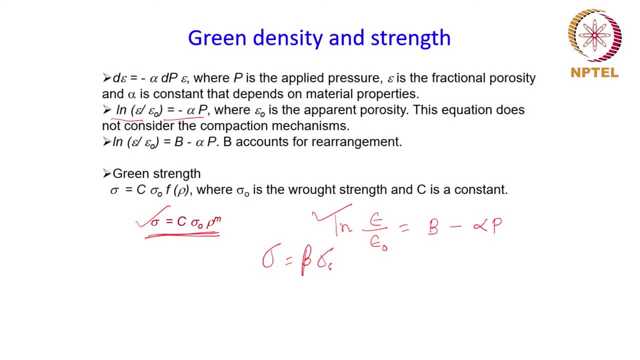 Where p is the compaction pressure, sigma 0 is the rot strength of the material and beta is a material dependent constant which also depends on the powder characteristics. So if you plot this equation, you will get a plot like this which will depict the real 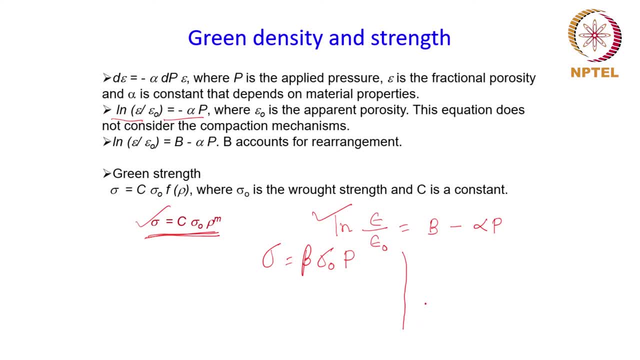 relationship between the green strength and the compaction pressure. The pressure is in MPa. So let us consider a particular powder, Just to demonstrate. So let us say we are talking about iron powder, which is irregular in shape, The green strength with respect to the compaction pressure will vary significantly. 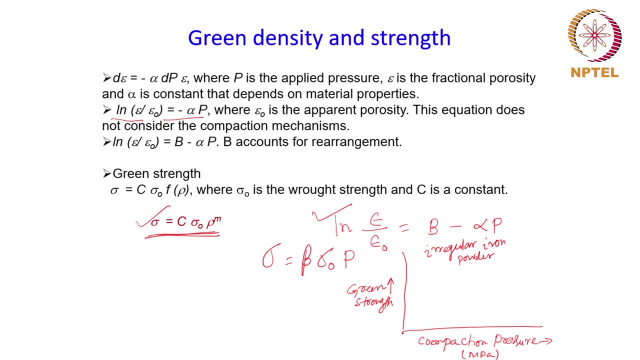 It will vary something like this. So at low compaction pressure there is a good correlation between this equation and the compaction behavior of the powder. but at higher pressure this does not really follow this equation, in the sense that the rate of compact strengthening is generally less than. 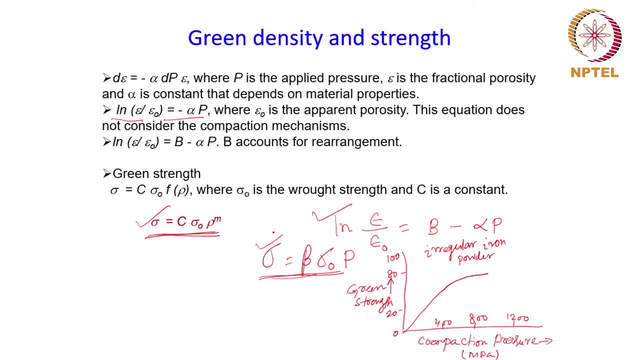 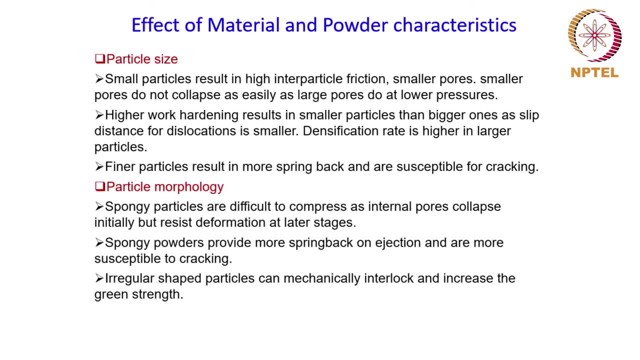 that will be projected by this particular equation. So, nevertheless, this plot will show a relationship between the compaction pressure and the green strength for a particular type of powder. So now let us see what is the effect of material properties and the powder characteristics. 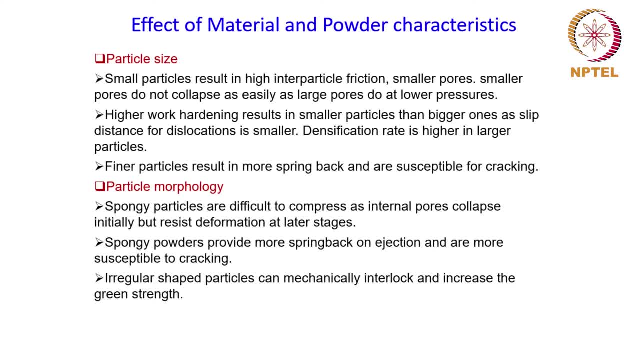 on the green density and the green strength of the compact. So let us first talk about the particle characteristics. So the two tote pode main particle characteristics which will have a bearing on the densification during the compaction process are particle size and particle morphology. 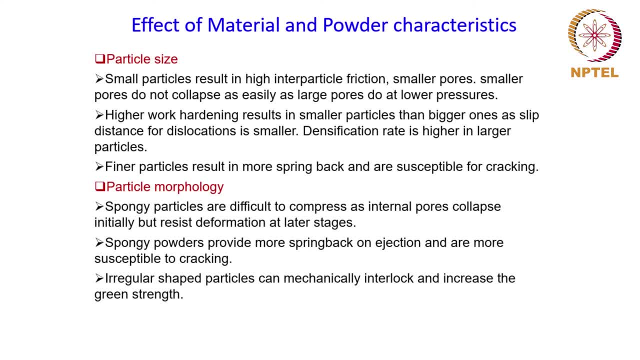 So, talking about the particle size, small particles will generally result in high inter particle friction and smaller pores. So high inter particle friction, as we have already discussed before, would actually hamper the packing of the particles, And small pores, on the other hand, do not collapse as easily as the large pores do. 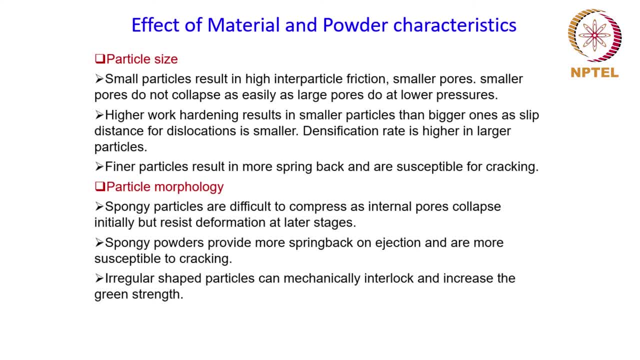 particularly at lower pressures, and therefore this will also hamper the green density that can be achieved at a particular pressure And the small particles also go through a higher work hardening because the slip distance for dislocations is smaller in smaller particles compared to the bigger ones And that will also result a lower densification rate. 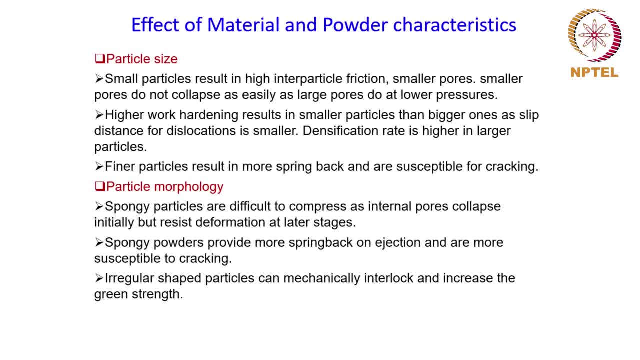 compared to larger particles. Now there is something called spring back that occurs when the compact is ejected at the end of the compaction process, right? So this is some recovery that happens in the dimension of the compact as it is ejected from the die. 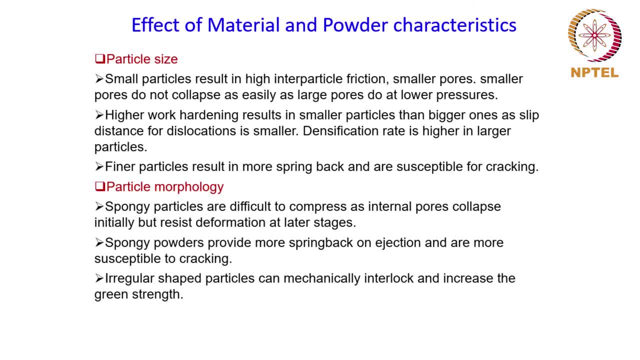 So finer particles will result in more spring back and are susceptible for cracking right. So when the spring back happens, if the spring back is larger or the recovery is greater, then there are chances that you know stresses will be developed in the compact. 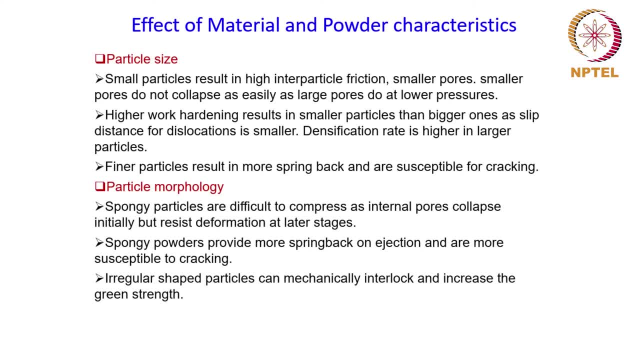 And it might even crack under those stresses. right And finer particles are more susceptible for this kind of cracking. ok, So this is how the compaction process as such and also the density of the compact which can be achieved are dependent on the particle size. 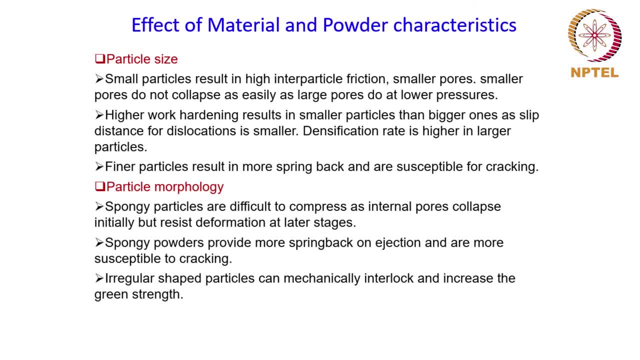 Now, when you talk about the particle morphology, we have seen there are different kind of morphologies generated by different fabrication routes which are used to process the metal powders. Spongy particles, for example, are difficult to compress as internal pores will collapse initially. 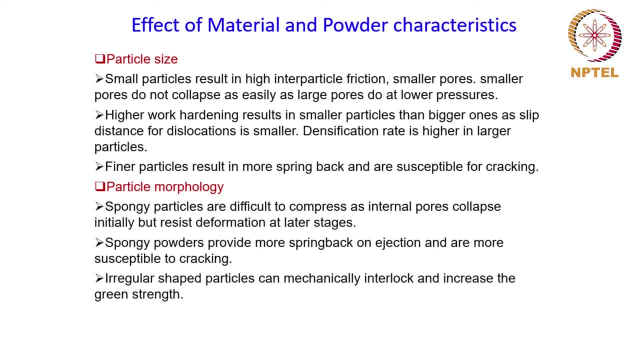 but resist the deformation at later stages, right? So this kind of spongy powders, as you might know, will have lot of porosity And as you apply the pressure, you will have a lot of porosity. So this kind of spongy powders, as you might know, will have a lot of porosity And as you apply the pressure, 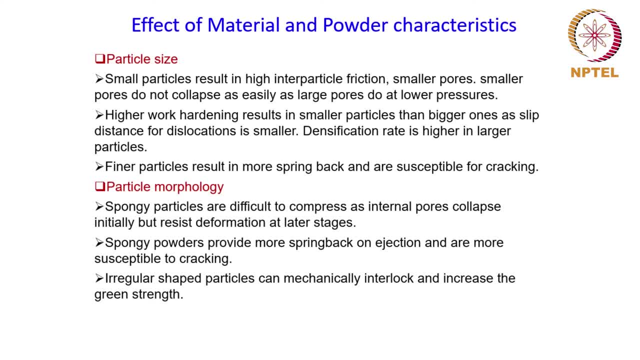 before the compaction and densification starts, this pore will actually start collapsing. ok, So the pressure will actually go into collapsing these pores rather than compacting the powder or densifying the powder. right, But as you progress, as the pressure is. 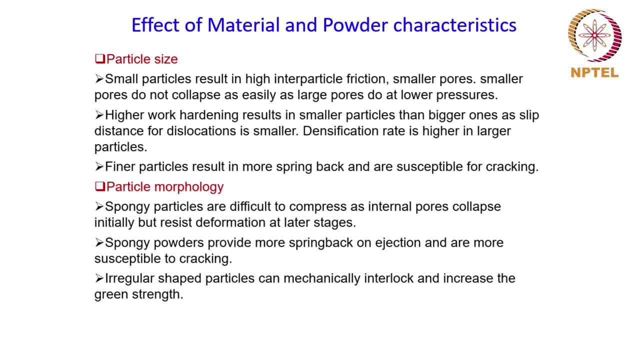 increased. the pores will also resist the deformation at later stages. ok And spongy powders will provide more spring back on ejection and therefore are more susceptible to cracking. Irregular shaped particles, on the other hand, can mechanically interlock and this will increase the. 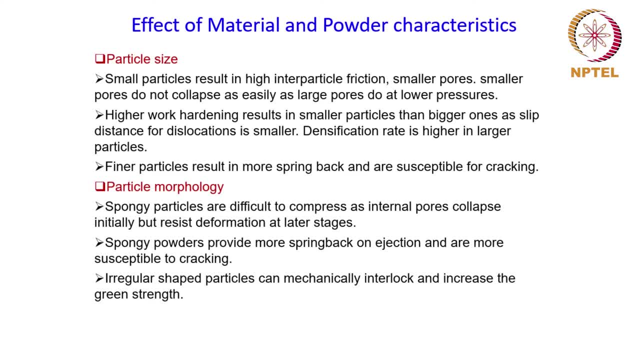 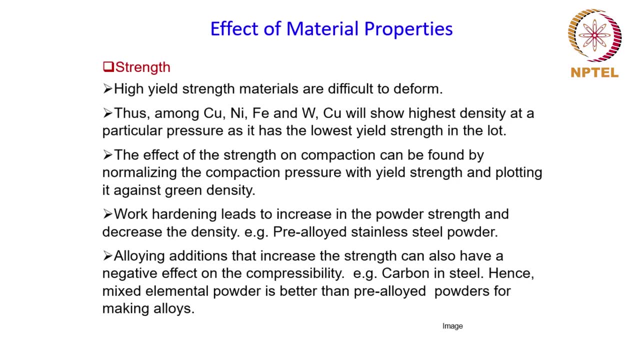 green strength. ok, So this is just an example of how the particle morphology will affect the compaction process and the green density. Now, when you talk about material properties and their effect on the compaction process and the green density, basically there are two material. 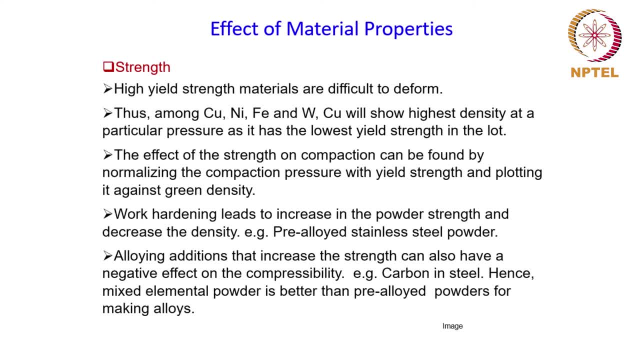 properties which will come into force over here. One is the strength and the other is the hardness, because these, these two are kind of related to the deformation behavior of the material And during the compaction, as we have seen, the powder goes through the deformation process. 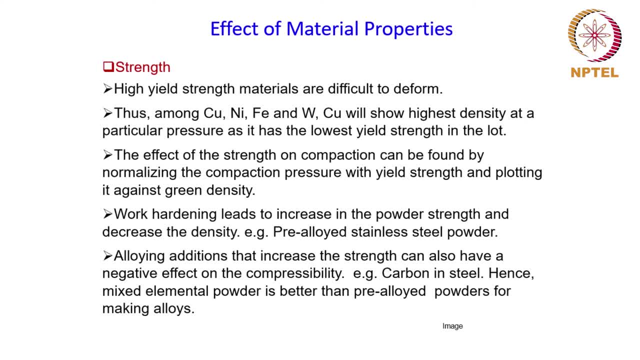 right. So anything which relates to the deformation process, we will have a bearing on the compaction process as well. So let us first talk about the strength and how it affects the compaction behavior of metal powders. So when the metal has high yield strength, 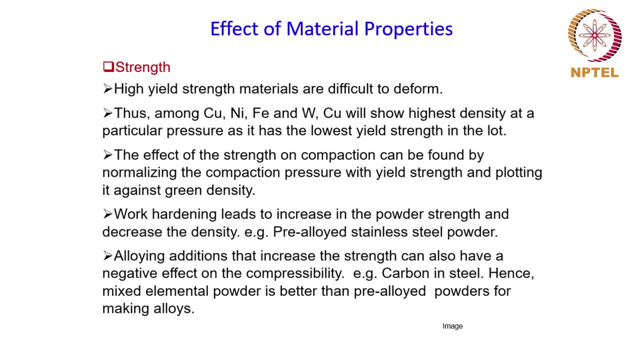 it will be difficult to deform, which is quite obvious. Yield strength is nothing but the stress at which the metal is produced, So that is what we will discuss today. So let us start with the. the material starts to deform plastically, So higher yield strength means you need a higher 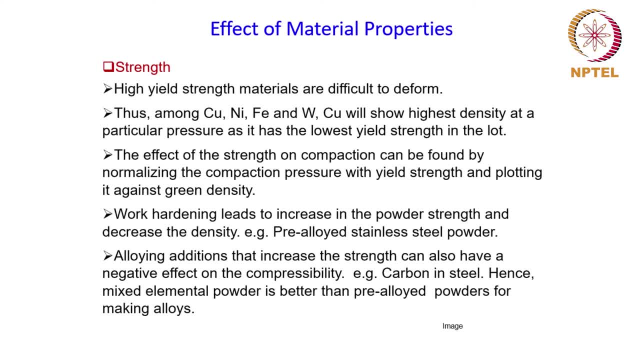 stress or a higher load to deform the material. And therefore, if you talk about materials like this and if you compare them, then the metal which is the lowest strength will give you the highest density at a particular compaction pressure. right. So if you talk about copper, nickel, iron and tungsten, copper will show the highest density. 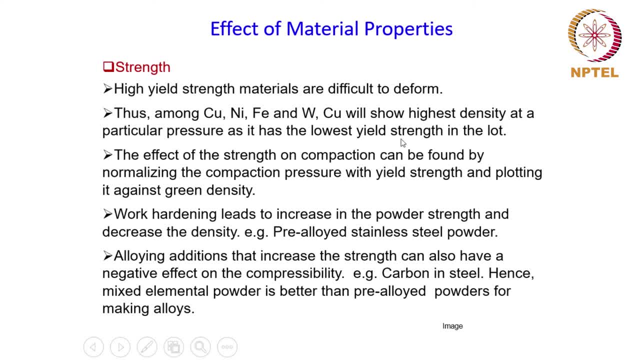 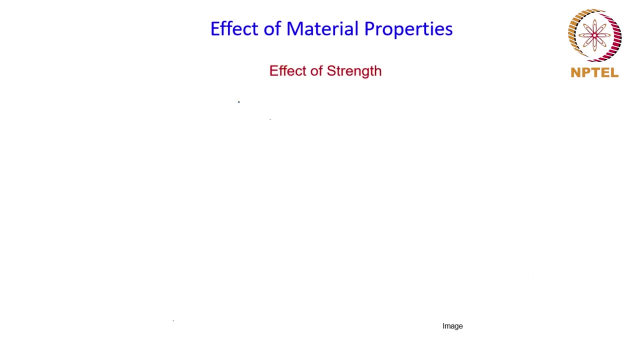 because it has the lowest yield strength, right? And this effect can be also shown graphically if you normalize the compaction pressure by yield strength and plot it against the green density. ok, So let us see how that plot might look like Battling. 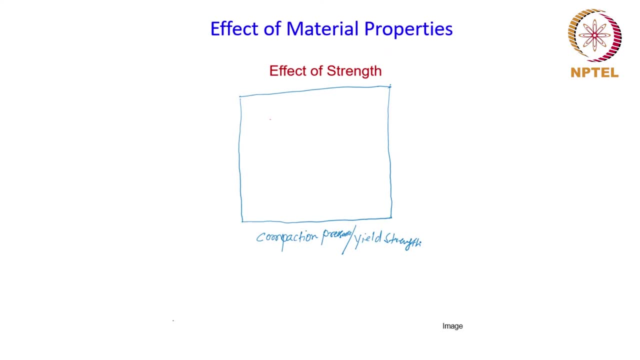 Gap at aaghya. So the x axis is the normalized compaction pressure and y-axis is the fractional density. So the plot might look like this. So the plot might look like this And, depending on the strength of the material, the data points may be below. 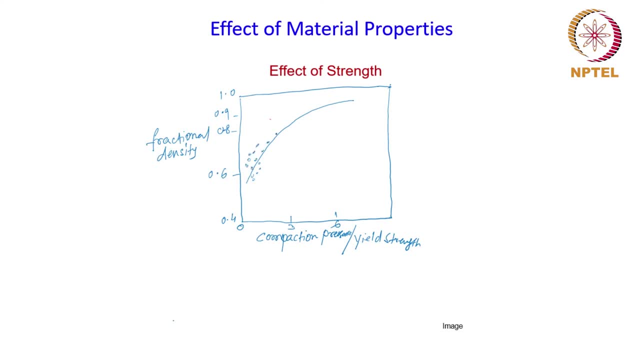 above or on this curve right. So, if you talk about a particular compaction pressure or a normalized compaction pressure, materials like copper will have points which are above because, as I said, at a particular compaction pressure, copper will have a higher fractional density compared to. 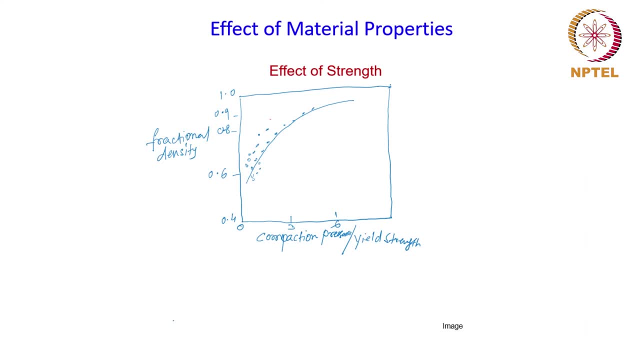 a higher strength metal like tungsten, And therefore it will lie above compared to the higher strength metals. So if you compare this set of materials, copper will always have a higher green density at a particular compaction pressure And with regard to the strength alloying elements will have. 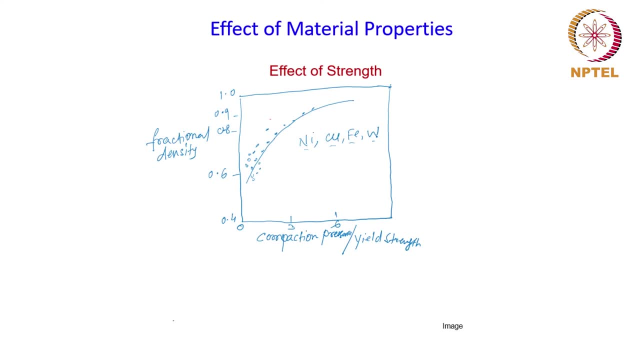 a very significant effect on the strength of a material. For example, if you talk about iron, If you add different alloying elements, the strength of the material will change and as a result of that, it will also affect the compaction behavior or the compressibility of the material. 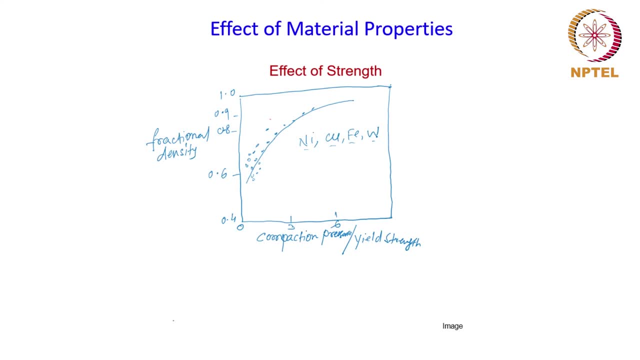 So, for example, if you talk about some of the alloying elements which are used in iron for making different grades of steel, such as chromium, molybdenum, nickel, manganese and carbon, uphouse is there If you see their effect. 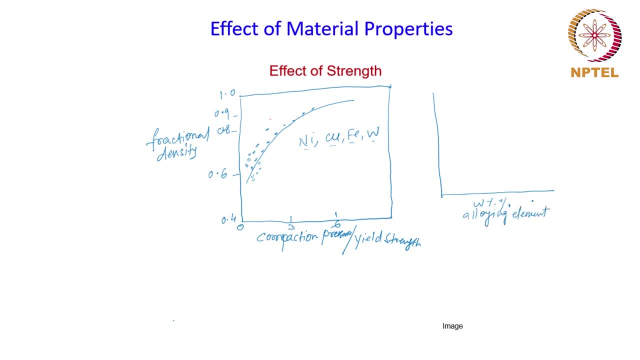 Let us say we are plotting the decrease in the compressibility against the weight percent of the alloying element. So the y axis is decrease in compressibility. So for different alloying elements the compressibility will change differently. For example, if you look at the y axis the compressibility of the alloying element will 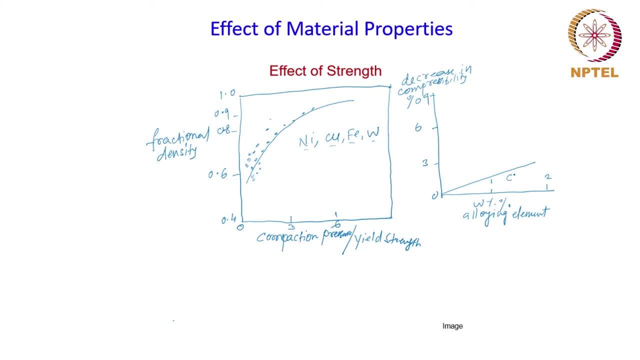 change. So, for example, if you look at the y axis, the compressibility of the alloying element will change. chromium it may look like this. Then, above this, you will have molybdenum, then nickel, then manganese and finally carbon. 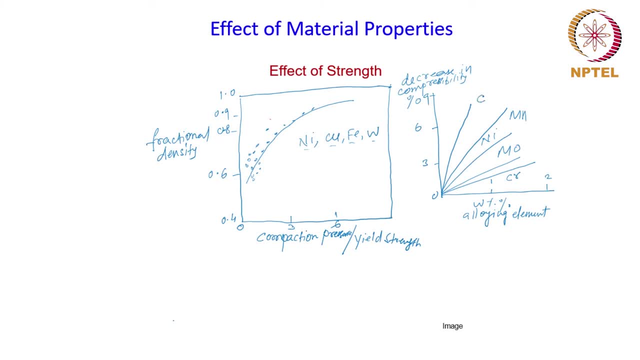 carbon. ok, So since all these alloying elements have their own effect on the strength of the material, they will also affect the compressibility or the compactability of the powder. We are talking about iron powder here. So the next important property which has a 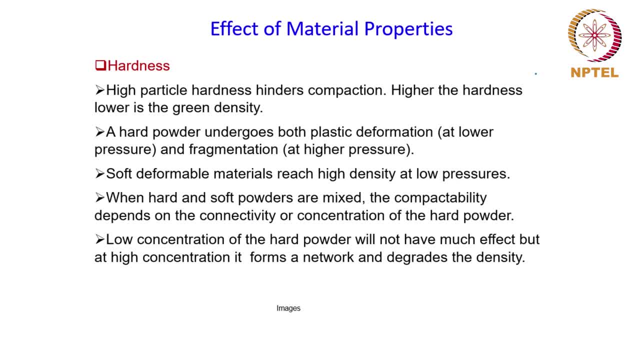 bearing on the compaction and the green density is the hardness. High particle hardness hinders compaction because, again, high hardness means it will have high resistance to deformation and therefore a higher hardness will be detrimental for the compaction process And therefore higher is the hardness. 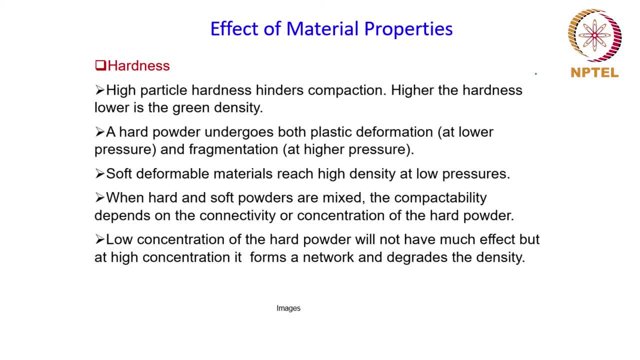 lower is the green density at a particular compaction pressure, And a hard powder will undergo both plastic deformation at lower pressure and fragmentation at higher pressure. ok, Soft deformable materials, on the other hand, will reach high density at low pressures because this kind of materials are easy to deform and they will easily form bonds with each other. 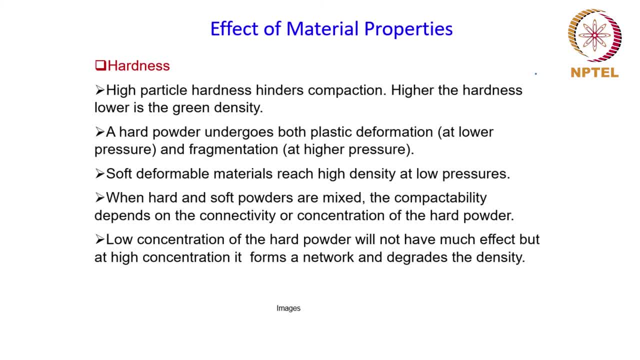 and therefore a high density can be achieved at lower pressures. Now, if you mix hard and soft powders, the compactability of this kind of mixture will depend on the connectivity or concentration of the hard powder. ok, So the hard powder will be dominating here in terms of deciding the compactability of that powder. ok, 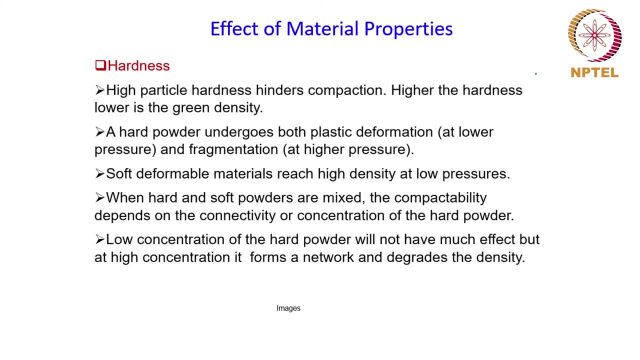 of the mixture. Low concentration of the hard powder will not have much effect, but when the concentration increases it will form a network, and this network of hard particles will degrade the density right, which is quite obvious because, as we have already seen, it is difficult to deform. 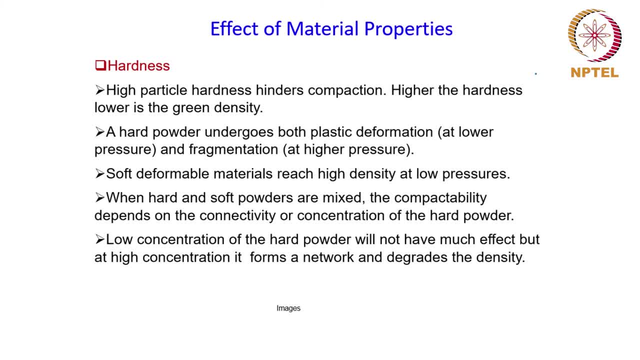 the hard particles and it is difficult to compact them, And therefore, if you have a network of this kind of hard particles in a matrix of soft particles, it will hamper the compaction of the soft particles as well and, as a result of that, it will also degrade the density of the compact. 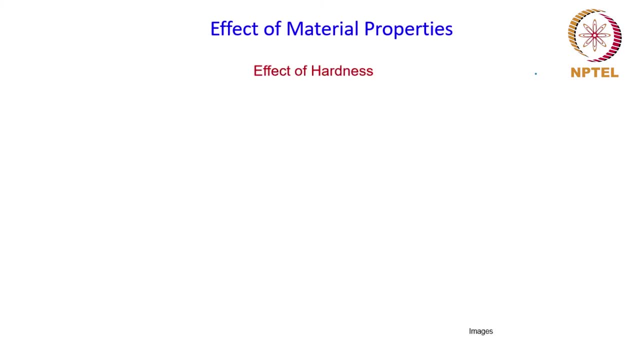 So we can take some examples and see how the material hardness affects the densification during the compaction process. So I will first draw a example of this picture of the hard particles. So the issue is that if we let us say we are plotting this at densification against the compaction pressure. 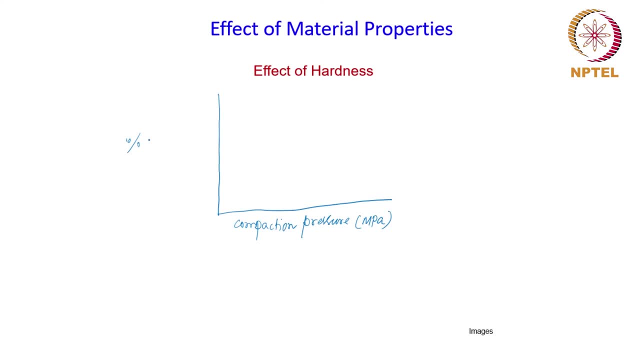 Thank you. Thank you, And we are talking about a powder particle size in the range of 44 to 62 micron, right? So, just to demonstrate this, we will choose some materials which are known for their high hardness and we will also choose some materials which are having much lower hardness compared. 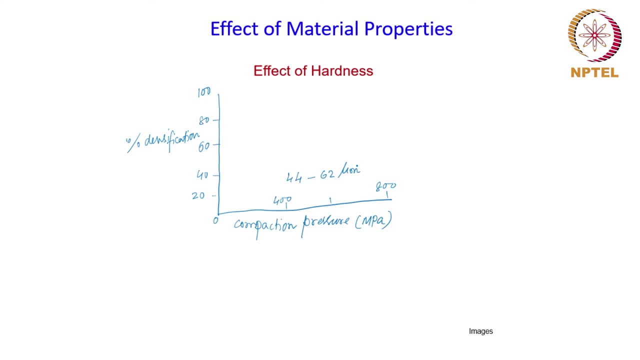 to harder materials right. For example, if you consider aluminium oxide or alumina, it has a new hardness of about 2100, and if you take a material like calcium carbonate, that is much softer compared to this aluminium oxide, since the hardness is only 135.. 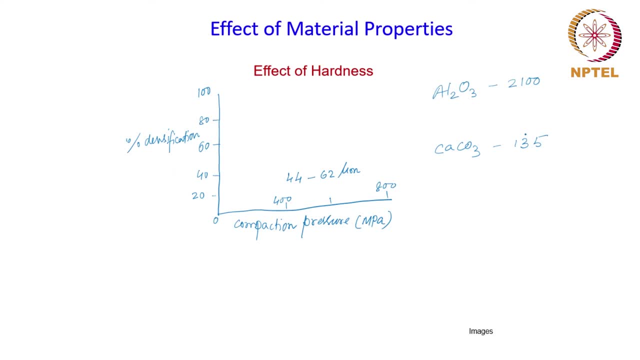 Ok, Ok, Then in between you may have silica, which is having a hardness of 820, magnesium oxide with about the hardness of 370, ok, So if you plot this kind of materials, ok, So if you plot this kind of materials, ok. 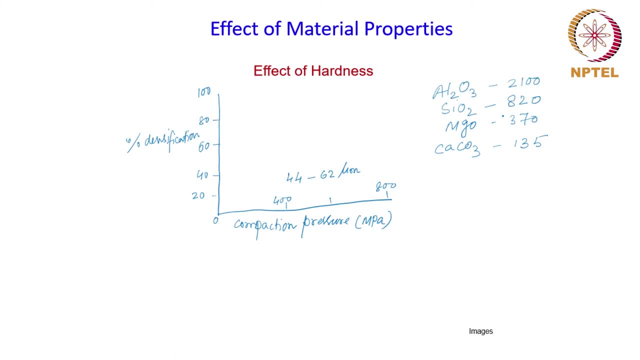 So if you plot this kind of materials, ok, Ok, So you will find that the curve for the calcium carbonate will be at the top, followed by magnesium oxide And finally at the bottom you will have it for aluminium oxide. ok, 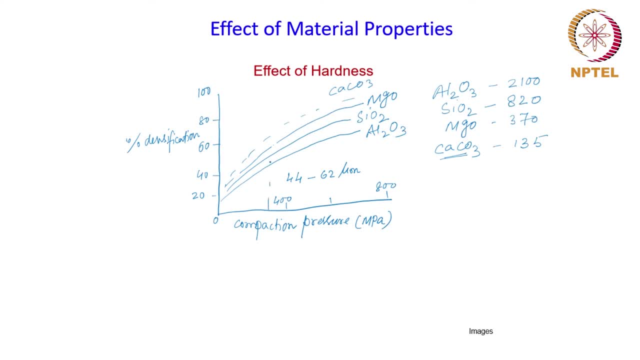 So this tells you that at a given compaction pressure, the density for the soft material will be always higher compared to the harder material, right? So in this pack, calcium carbonate is the softest and therefore, at any given compaction pressure, the densification or the fractional density will be highest for the calcium carbonate. 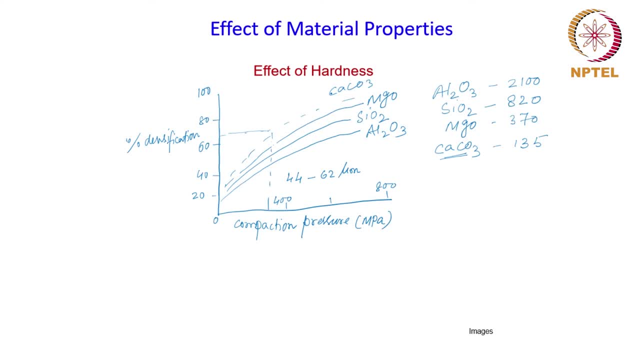 and aluminium oxide is the hardest in this pack and therefore it will have the lowest density at a given compaction pressure. Ok, right, So that is how you can see the effect of hardness on the densification which happens during compaction. ok, So before we finish this class, let us take 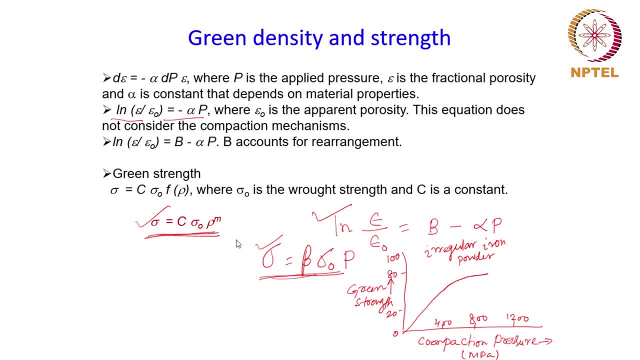 a moment to summarize it. Today, we learned about the correlation between the material properties and the green density, or the densification during compaction. We have also seen how the green strength depend on the compaction pressure, with the help of a plot like this. So you? 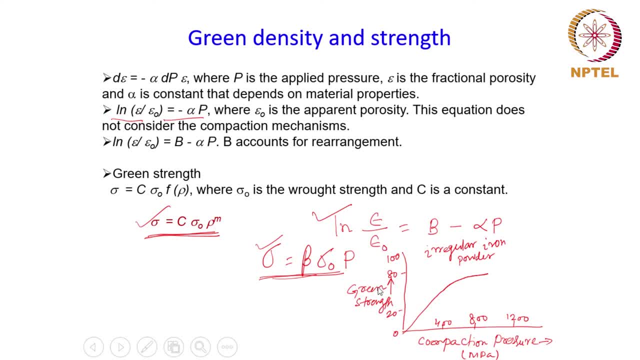 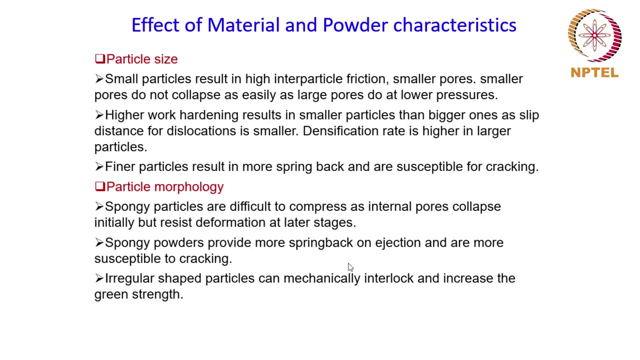 can see, as the compaction pressure increases, the green strength will also increase, which is obvious, And we have also derived an empirical equation for that. This equation correlates the green strength to the compaction pressure p. Then we talked about the effect of particle characteristics on the densification process, And here we 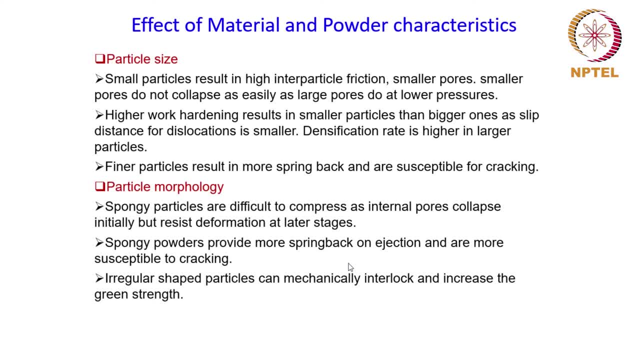 talked about two characteristics of the particles- One is the particle size and another is the particle morphology- And we have seen that it is difficult to compact smaller particles compared to the larger ones, and the primary reasons for that are as follows: inter particle friction is high for the smaller particles And they also go. 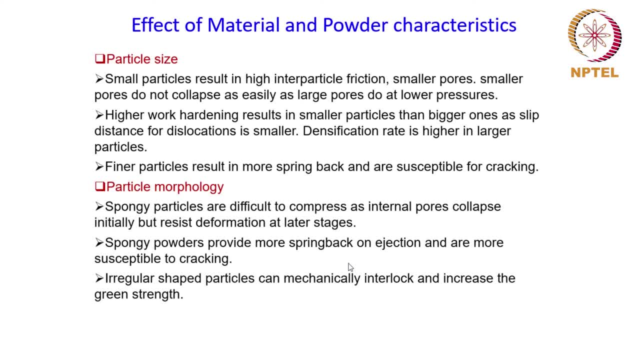 through a higher work hardening compared to the larger particles. So this particular equation obviously can be applied with some crimes. we have seen that wall hiding is also 치chi, So we know that the government into a such a state where this 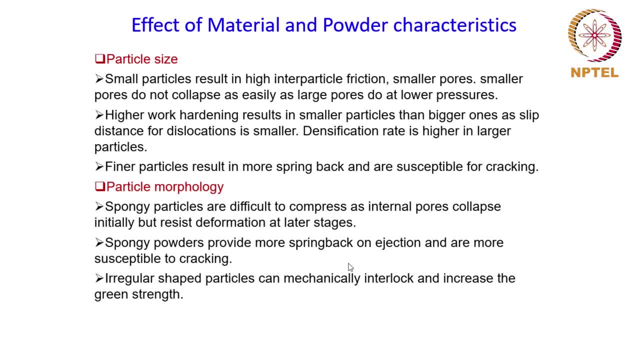 concentrated, much of the Goodman area of the brown cell lines come up. So now the product is a large particle, the solidium, and the increases are changing as they go along with the And they result in more spring back and are also susceptible for cracking ok. 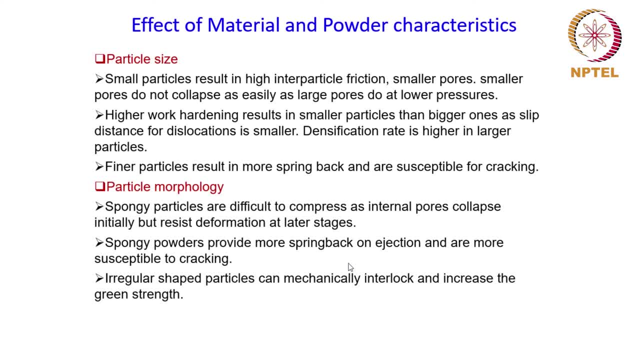 So, due to all such characteristics of small particles, they are difficult to compact compared to larger particles. And in terms of the particle morphology, we talked about two kinds of morphology: one spongy kind of morphology and another was the irregular shape. 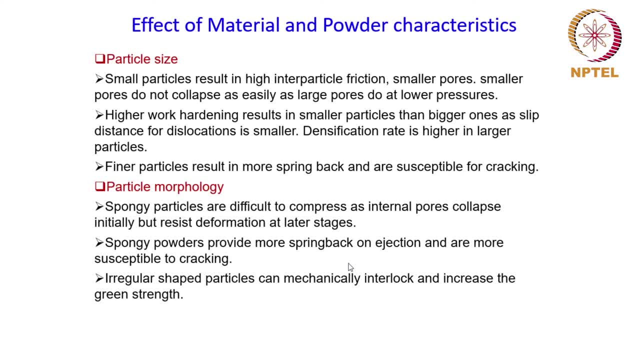 In case of the spongy particles, because of the presence of lot of internal pores when the powder is pressed. these pores will collapse in the beginning, but ultimately they will resist the deformation at later stages, And this kind of spongy powders also lead to more spring back on ejection at the end. 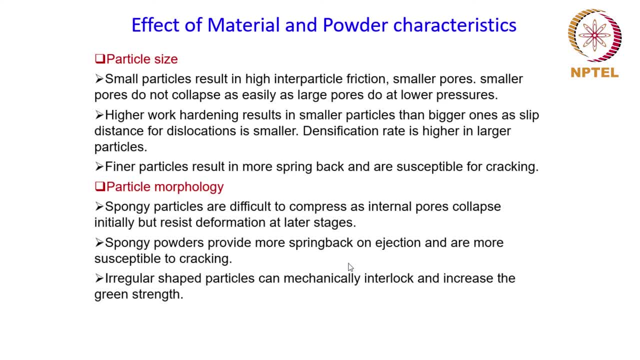 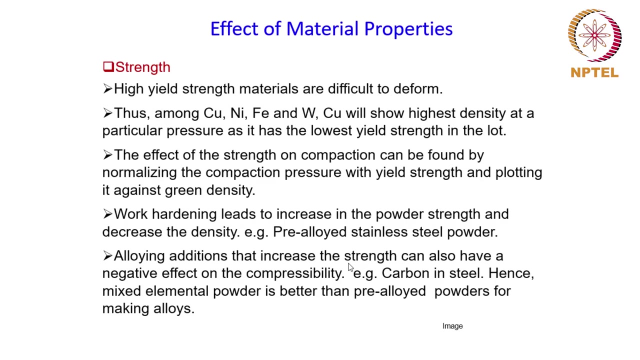 of the compaction process and are also susceptible for cracking. Irregular shaped powders, on the other hand, can mechanically interlock and hence increase the green strength of the compact. Then we talked about the effect of the material properties on the densification process, as 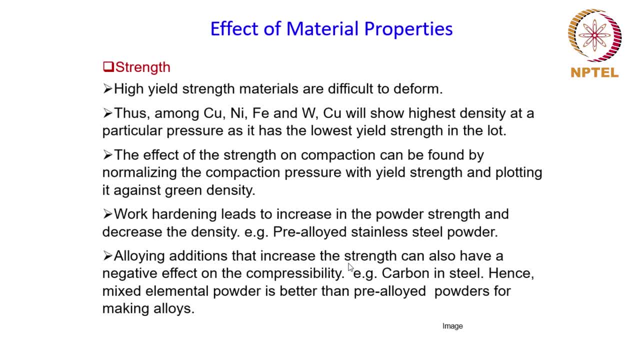 it happens during compaction And we have seen if the material has highest strength or higher yield strength, it will be difficult to deform compared to a material which is having lower yield strength. And this we have also demonstrated with the help of a plot like this: 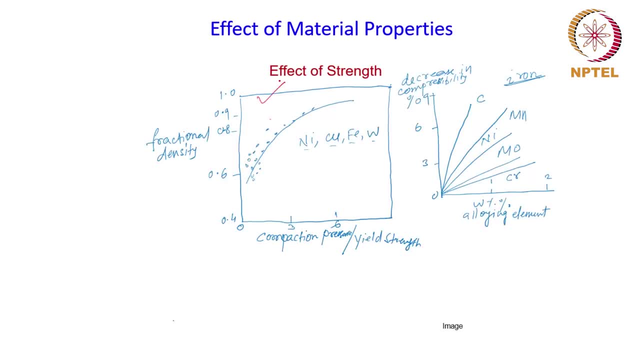 So we have seen the effect of the material properties on the densification process, as it happens during compaction, and we have seen if the material has higher strength or higher yield strength. This is which shows the correlation between the fractional density and the normalized 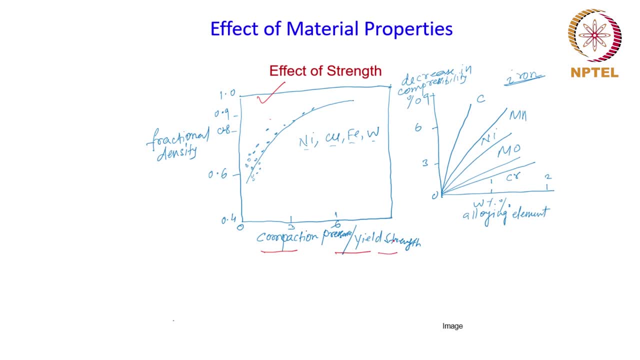 compaction pressure. The compaction pressure is normalized with the yield strength of the material And we have seen a lower strength material like copper is easier to compact and will have higher fractional density compared to a higher strength material- strength material like tungsten or iron. Then we also talked about the effect of 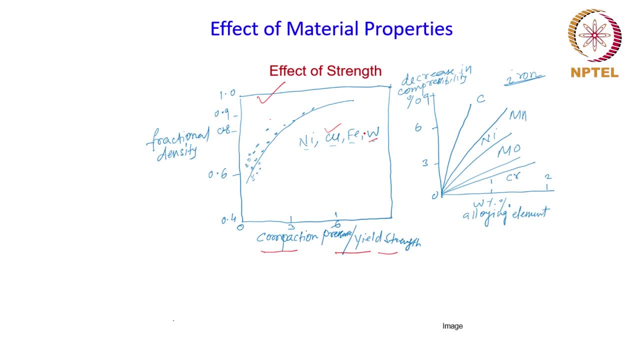 the alloying elements which influence the strength of the material, and we took this example of iron and different kind of alloying elements which are added to iron for making different grades of steel. So they will also have their own effect on the compressibility, since they affect the strength of the material.